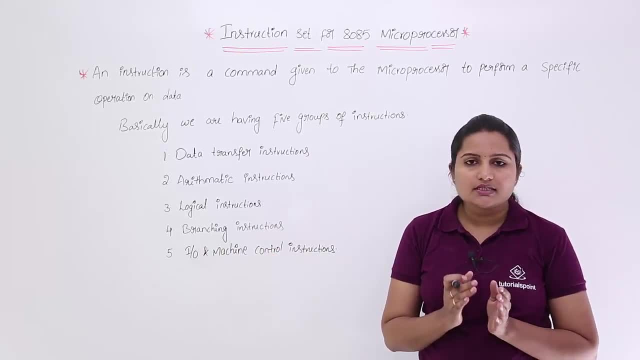 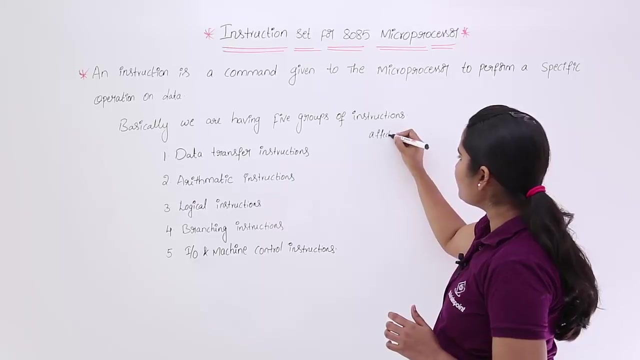 So now coming to IO and machine control instructions, these are some special instructions, So in this the instructions contain IO and machine related contents. So here coming to the effect of flag flags, effect on flags. so that means the effect of these instructions on flag Favoritism. 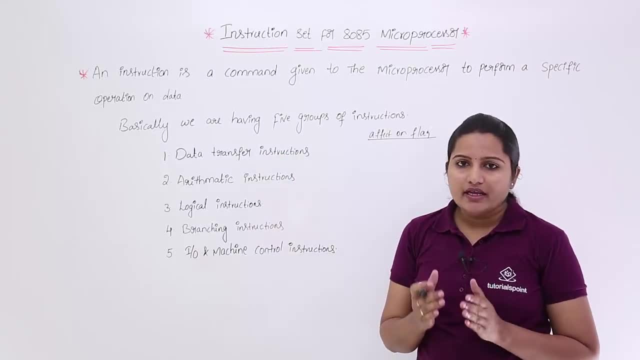 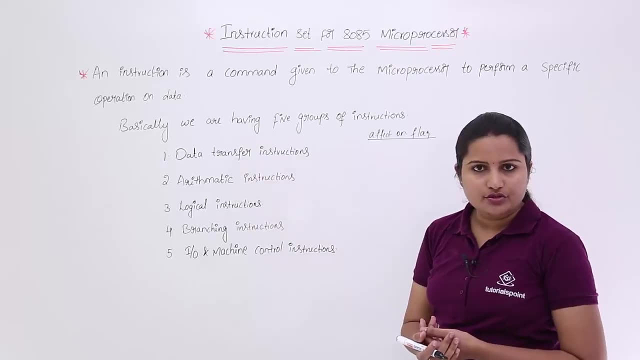 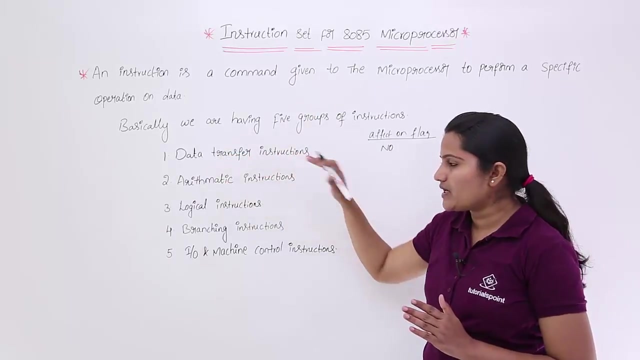 So, coming to data transfer instruction, when we processed this instruction. so then, when we executed this instruction, then no flags are going to affect. So, after execution of this data transfer instructions, so no flag register, no flags of flag register are going to affect. So no problem for flag register by data transfer instructions. 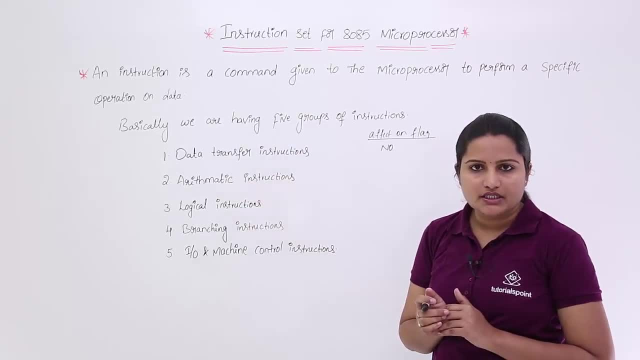 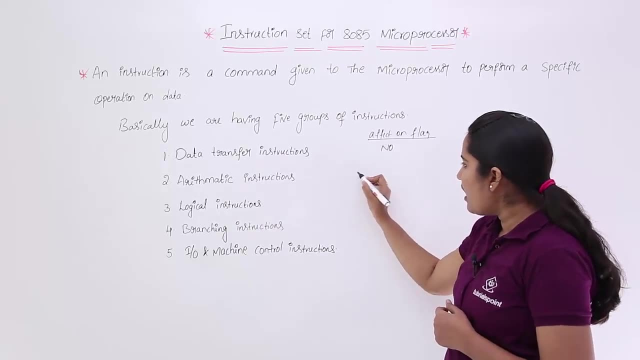 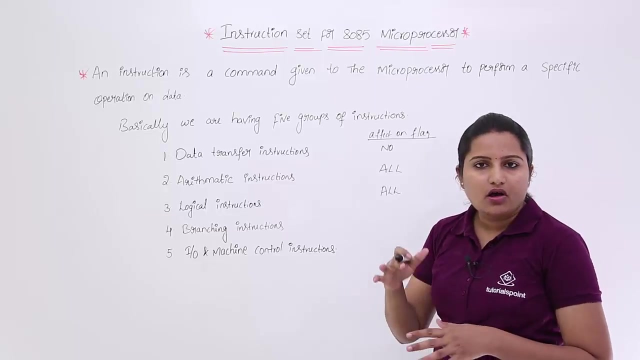 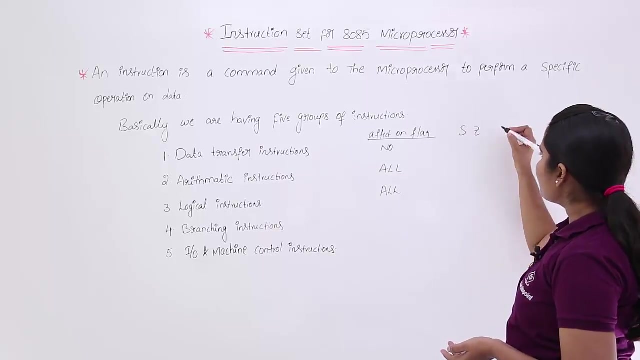 So now coming to arithmetic and logical instructions. So in arithmetic instructions, due to arithmetic instructions and logical instructions, almost all flags are going to affect. That means so for all arithmetic instructions all flags are going to affect. So how many flags we are having means sign flag, zero flag. so parity flag, auxiliary, carry flag and carry flag. 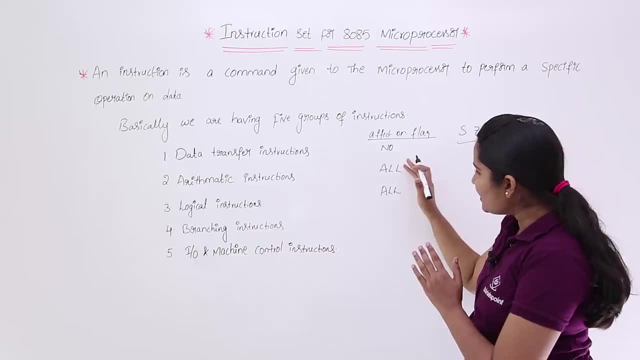 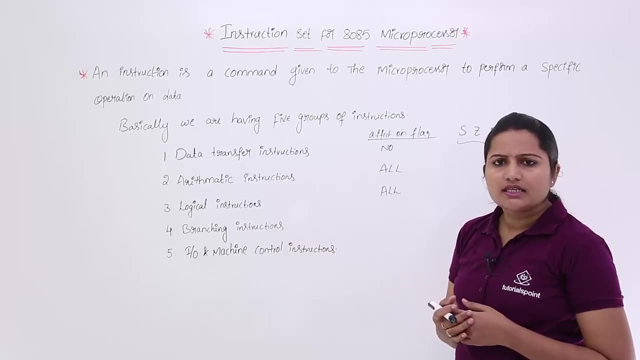 5 flags are going to affect there in flag register. So all these flags are going to affect by arithmetic instructions as well as logical instructions. Some logical instructions are there in which only some flags are going to affect, So but 99 percent of logical instructions due to that logical 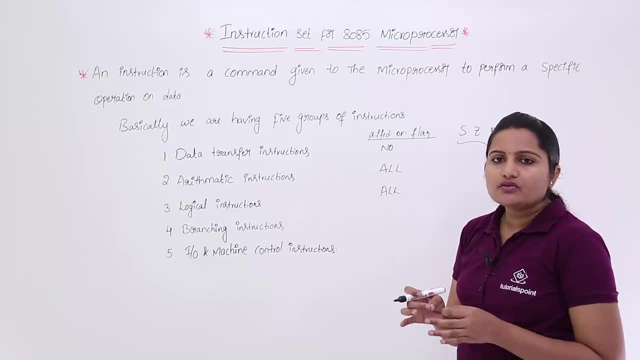 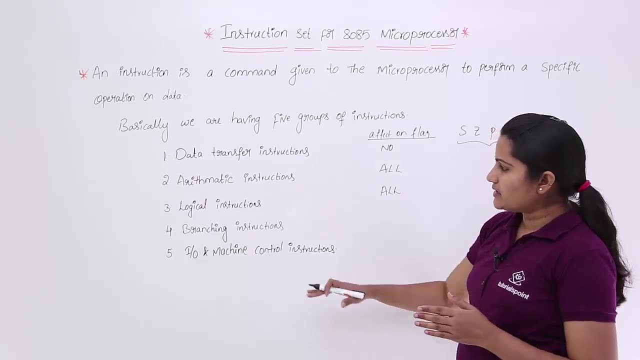 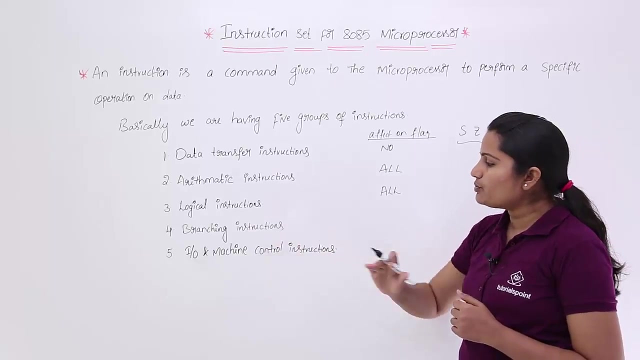 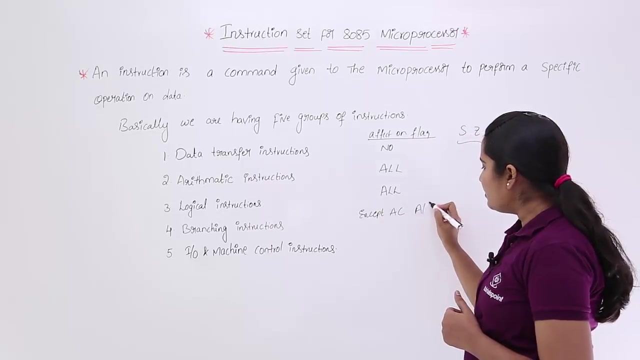 instructions all flags are going to affect. So I will tell you what instructions in logical instructions will affect minimum flags. So when we are discussing individually then we will discuss everything about flag registers effect and everything we will discuss there. and coming to branching instructions, except auxiliary carry flag, all flags are going to. 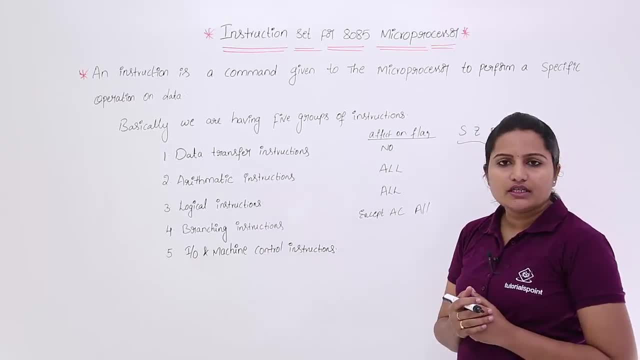 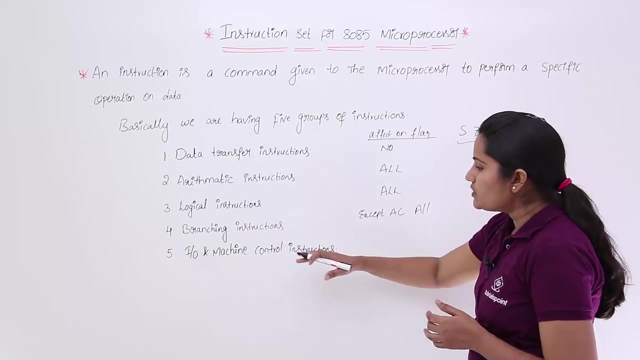 affect. So now coming to I, O and machine control instructions, due to these instructions, So which flags are going to affect means. So that is related to the instruction itself I will discuss when I am discussing I, O and machine related instructions. So coming to the flag affect. So here that is related.